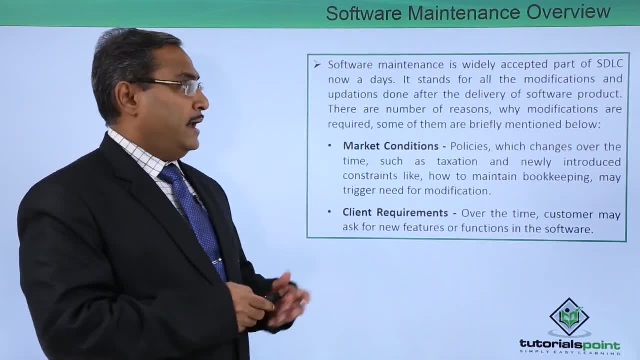 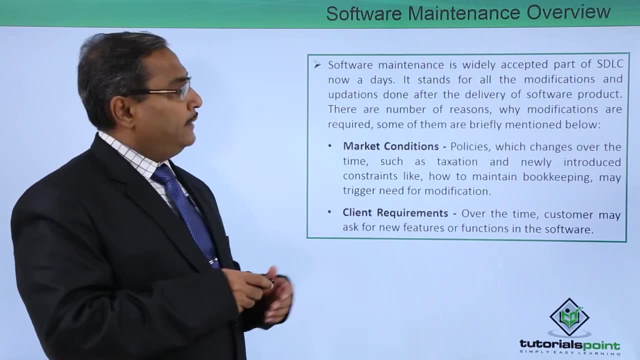 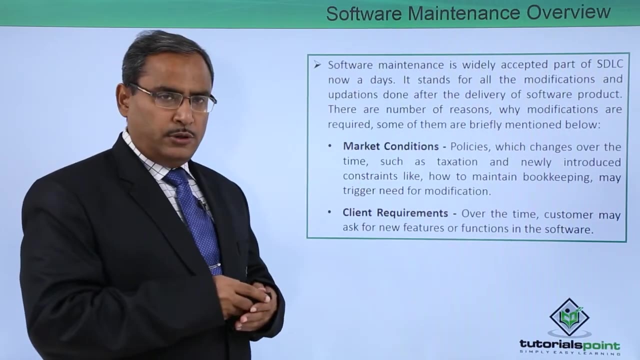 accepted part of SDLC nowadays and it stands for all the modifications and updations done after the delivery of the software product. And there are number of reasons why modifications are required, and some of them we have listed below. So let us go for the respective causes. 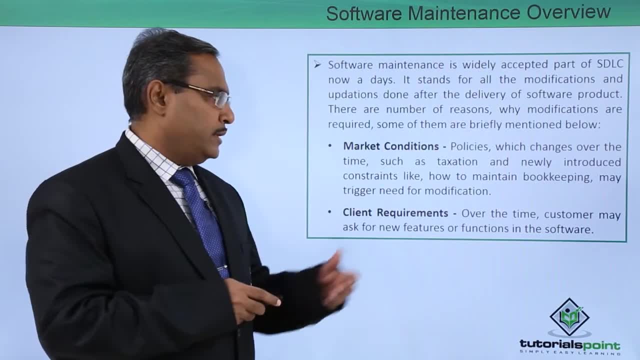 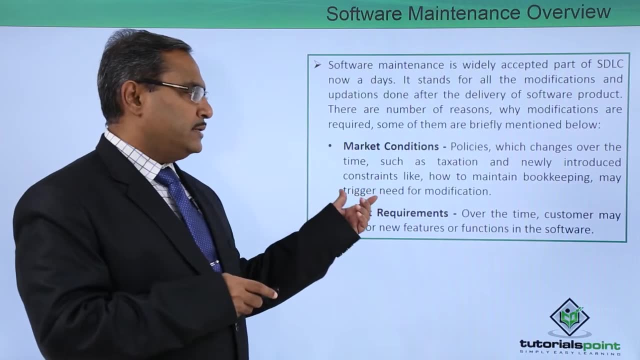 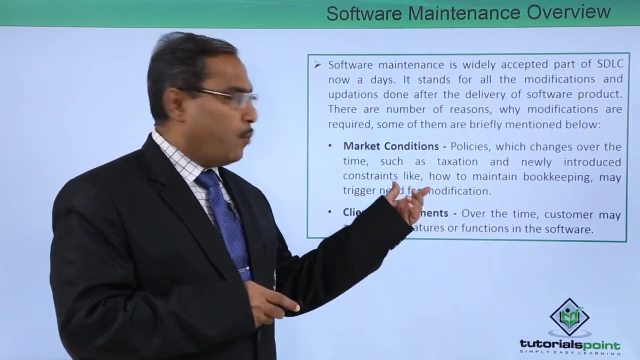 So the first one we are considering is the market condition. So policies which changes over the time, such as taxation, newly introduced constraints like how to maintain book keeping, main trigger, may trigger need for the different modifications. So that is why, due to the change in the government, 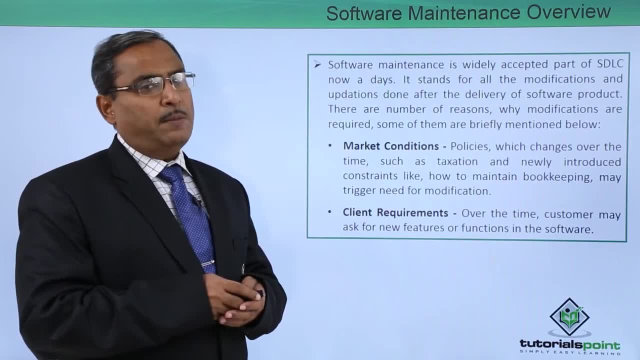 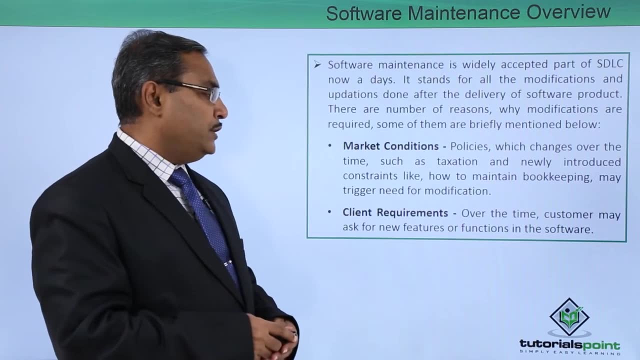 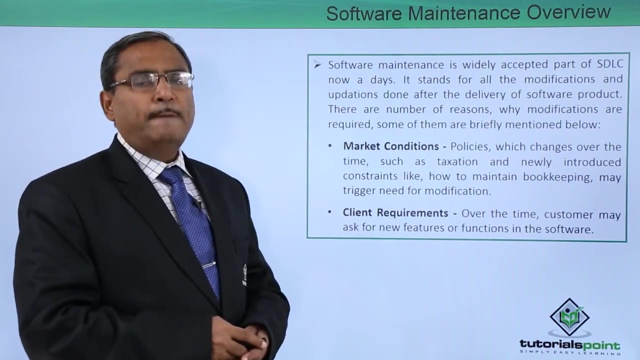 policy. due to the change in the market conditions, the maintenance might be required. Next one is our clients recommend. So over the time the customer may ask for new features or functions in the system to get implemented and incorporated. In that case also the software maintenance will be required. 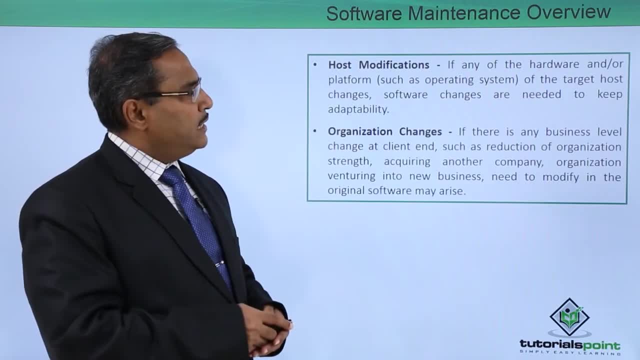 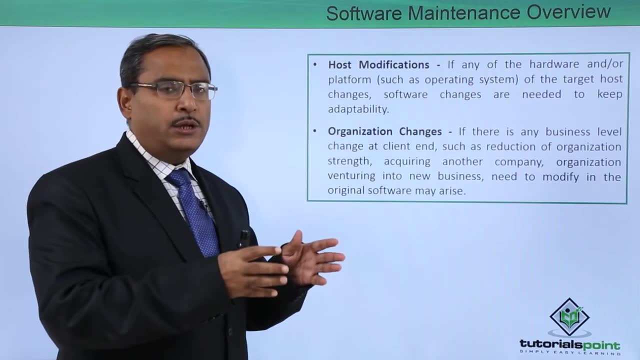 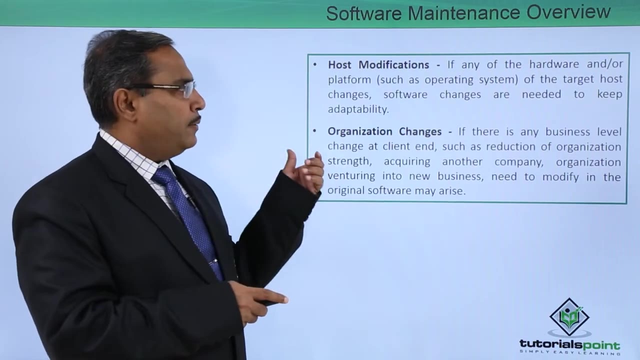 So next one: we are going for host modifications. So if any one of the hardwares and or the platforms, platform means actually the hardware and the operating system collectively, we usually call it as platform. So if any of the hardware and or the platform, such as the: 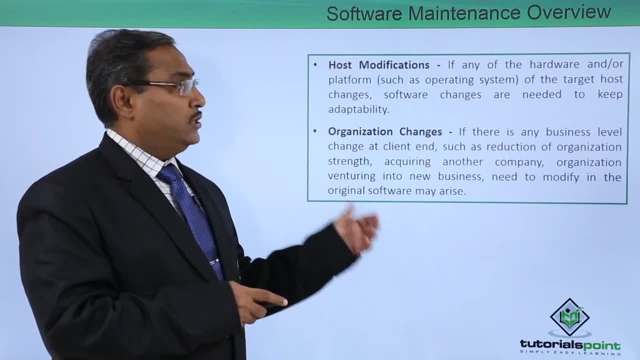 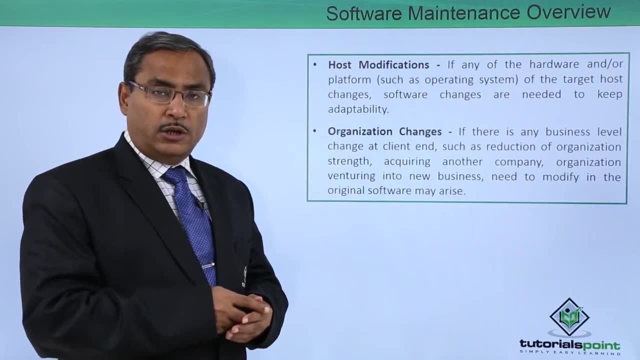 operating system of the target host changes. the software changes are needed to keep the adaptability and that is why the maintenance will be required. So there is some change in the hardware, there is some change in the operating system, there is some change in. 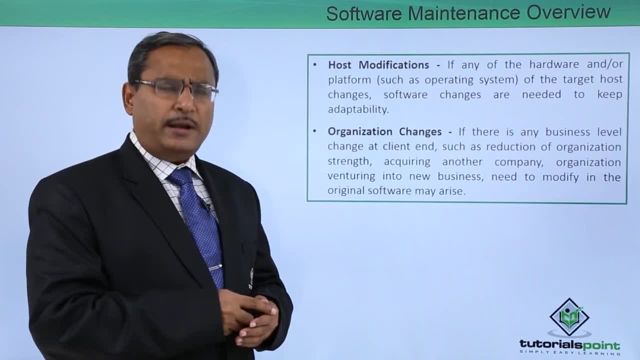 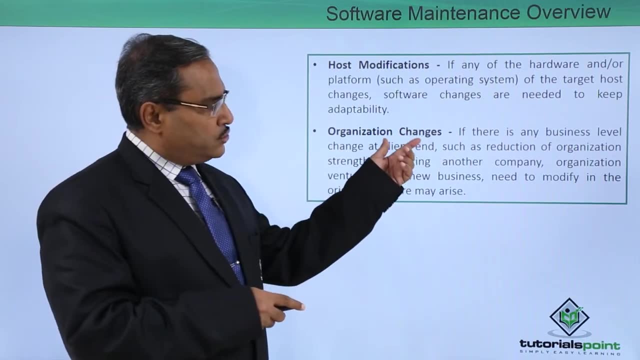 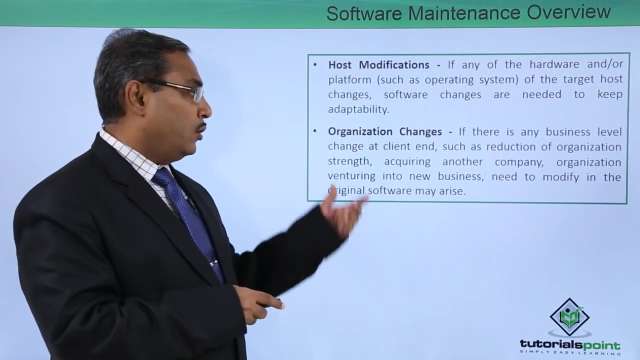 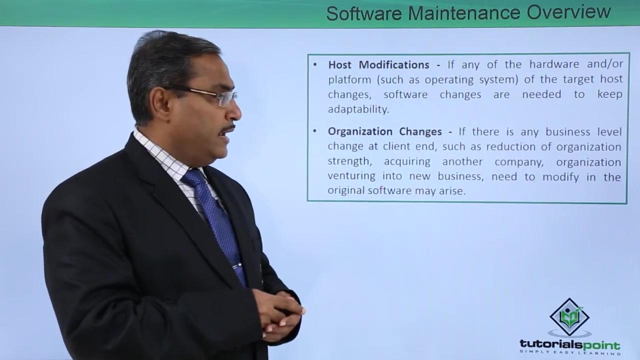 the respective drivers. So in those cases the software maintenance might be required. Next one is the organizational changes. So organization changes. so if there is any business level change at the client end, such as the deduction of the organization strength, acquiring another company, organization venturing into some new business need to modify in the original. 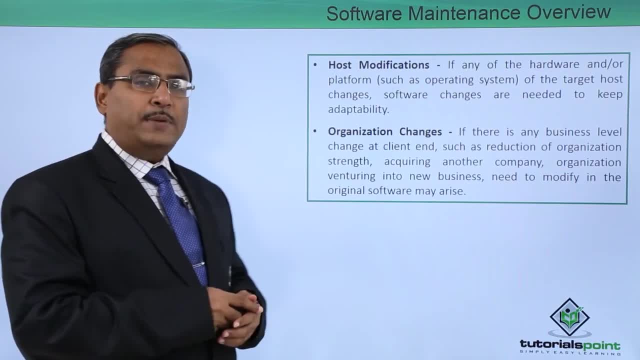 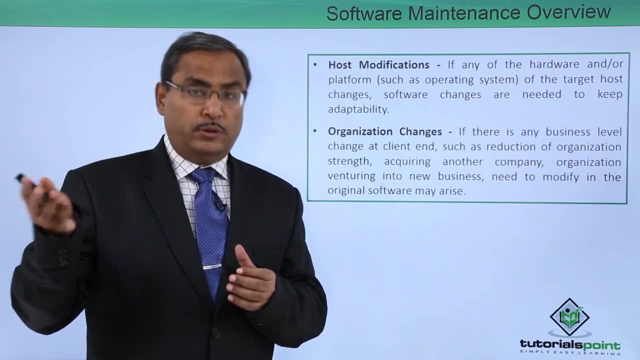 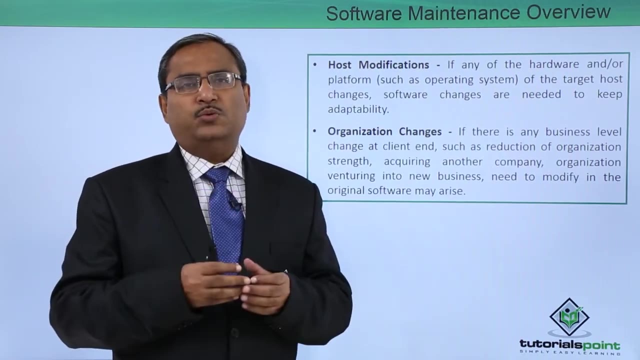 software may arise. So sometimes a company may be growing, sometimes a company may be shrinking, sometimes a company may be opening a new wing in which business they were not there previously. So, due to some reasons, the organization changes will be there and 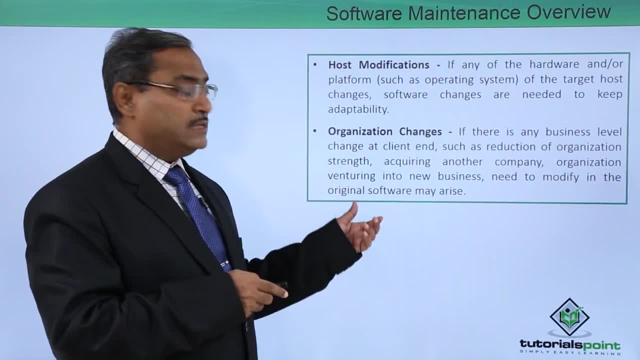 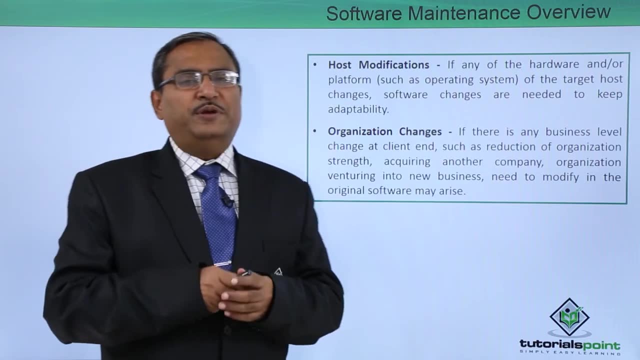 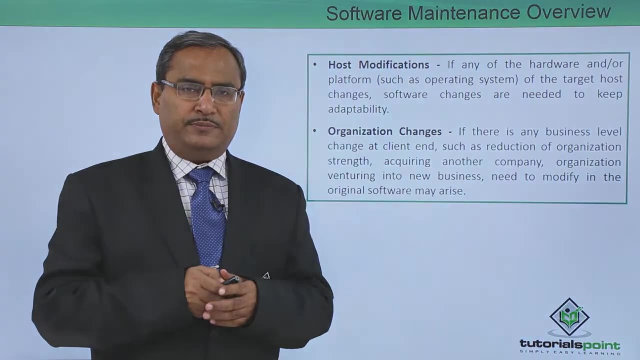 for that this software changes will be. some changes in the software will be there. So in this way, in this particular video, we have discussed what are the different software maintenance overview. Thanks for watching this video. 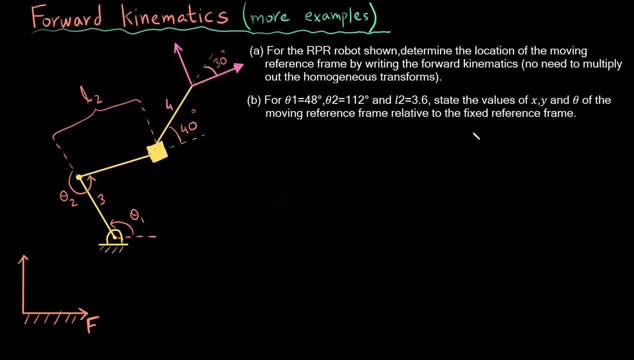 Hi, this is Zain Khan, here and now we are going to do an even more interesting example of forward kinematics. Before we move on to the question, let me walk you through the robot and a few things that you should know right away. So the first. 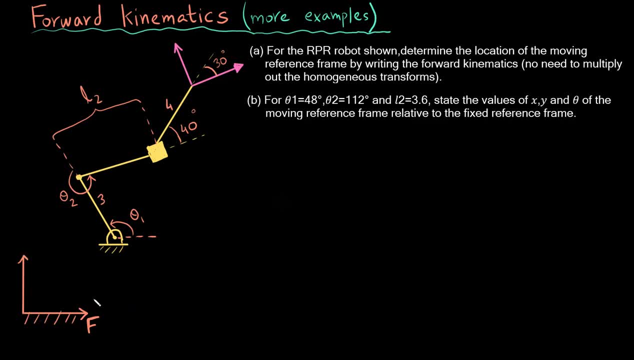 thing that we should know right away is that the fixed frame is not at the base of the robot, but it is placed somewhere here. So it is not at the base of the robot, but it is placed at a distance somewhere. It is given in the question. 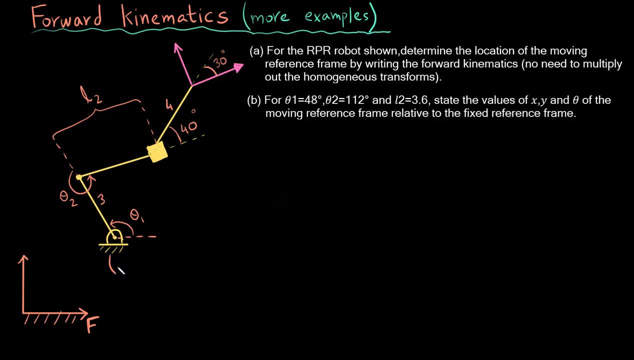 that this is displaced: four units in X and two units in Y. Now, the second thing that I need to note is that this robot is a RRP robot. What this means is that there is a revolute joint here and there is a revolute joint here, So there is going to be a motor attached at this. 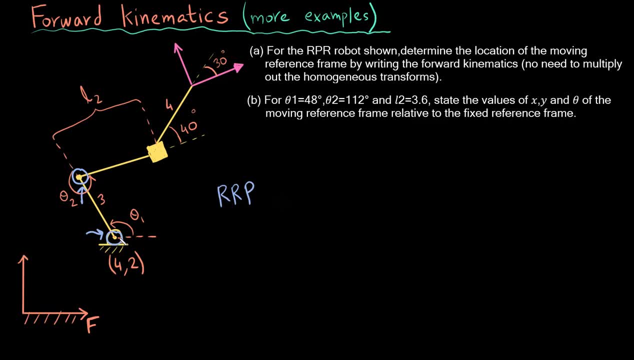 joint, and at this joint which allows the links to rotate, and then there is a prismatic joint at this point. So what it means is that this length right here is not fixed, but it can increase or it can decrease, since it is a prismatic joint.